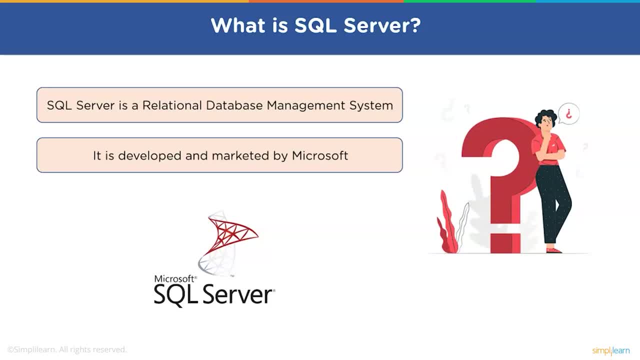 key, foreign key and other kind of integrity constraints you can maintain in this relational database. SQL Server is developed and marketed by Microsoft, So this is a Microsoft product, but it is compatible with all the technologies which you want, which you might be using or you might want to use, like Nodejs, Java, etc. where you want to connect your 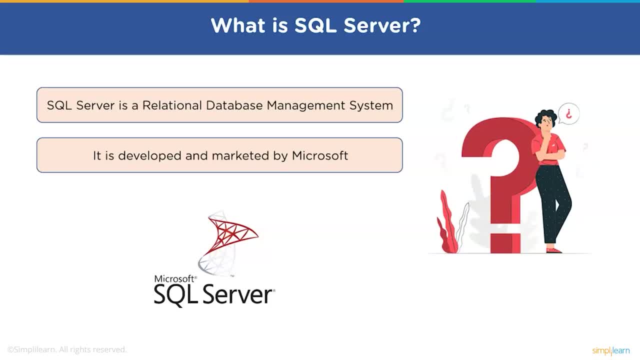 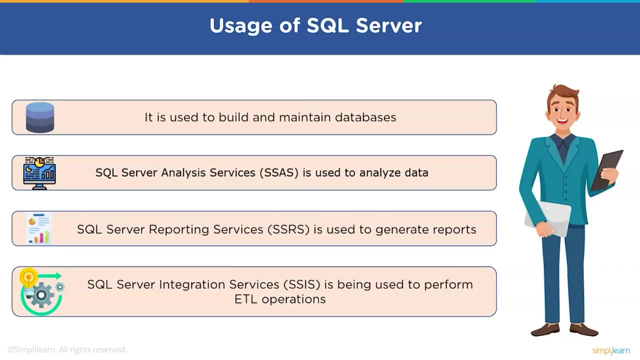 middleware application server with Microsoft SQL Server. Now, what is the usage of SQL Server? Apart from the definition which I just shared with you, for maintaining and building databases, persistent databases, there are other usages also, which I'll explain you Now. the first one is SQL Server Analysis Service, which is used to analyze data. Now the SQL Server. 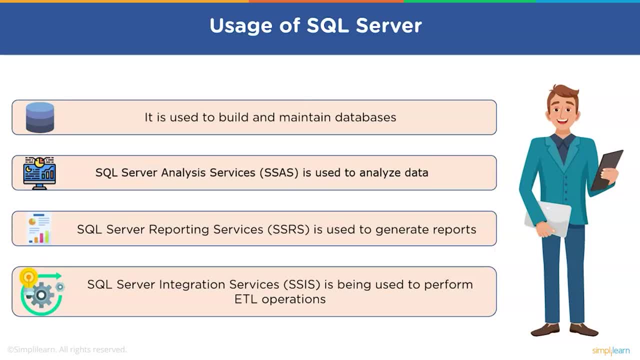 Analysis Service, or SSAS, is a multi-dimensional analysis tool that features online analytical processing, provides powerful data mining capabilities and deeper dimensions to business information within a relational database. Multi-dimensional analysis is an online analytical processing technique- OLAP technique- that produces the ability to analyze large quantities of data by storing data. 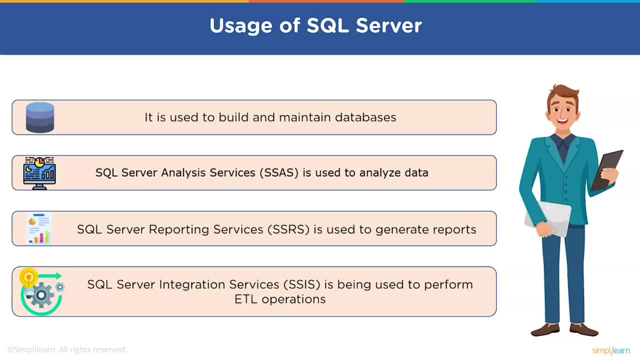 in axis and cells instead of traditional relational two-dimensional view in rows and columns. SSAS places predictive analytic capabilities in the hands of information workers by creating an instant connection to back-end data using familiar applications such as Microsoft Excel, SharePoint, etc. for analysis, visual representation and collaboration. The next is SQL Server Reporting. 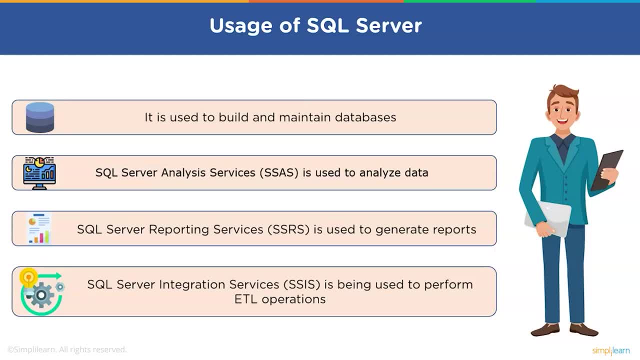 Services which is used to generate reports. Now, SSRS is a framework of reporting mechanisms such as the Report Builder, Report Designer, Report Manager and Report Server that work together through a web interface to enable the development of concise interactive reporting solutions in print or web format. Report Builder and Report Designer are two SSRS components for generating 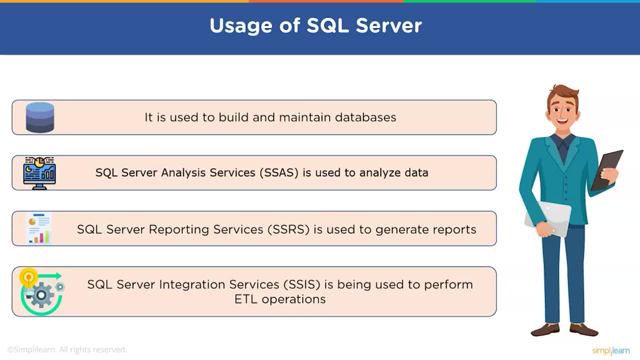 reports. Report Builder is a simple solution for the information worker or business user to create quick reports. The report designer is a tool for developers because it adds complexity to custom reports development and you create data models in it. Using this tool requires an understanding of. 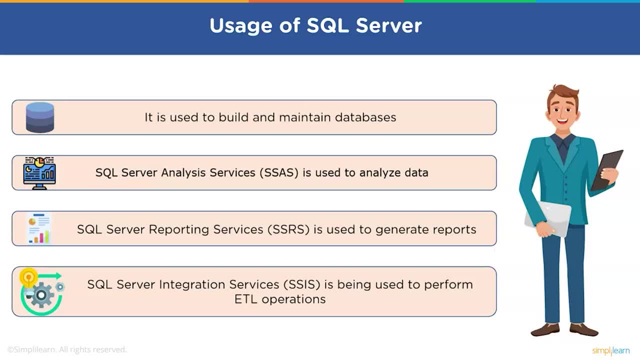 the Business Intelligence Development Studio shell in Visual Studio and the underlying structure of the data, so you have to be aware of it thoroughly. According to Microsoft, the report server is the SSRS that manages the processing and delivery of reports using processors. The report manager is: 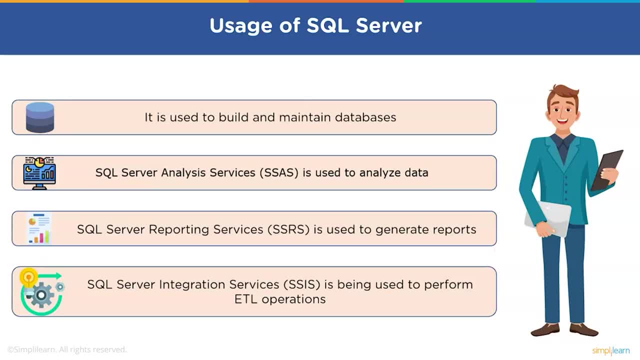 an administrative tool that controls reporting services through a web interface. Now let's talk about another important component, which is SQL Server Integration Services, SSIS, which is being used to perform ATL operations. Now, SSIS is the data arm of the SQL Server equipped with Superior Extract, Transform and Load Capabilities. 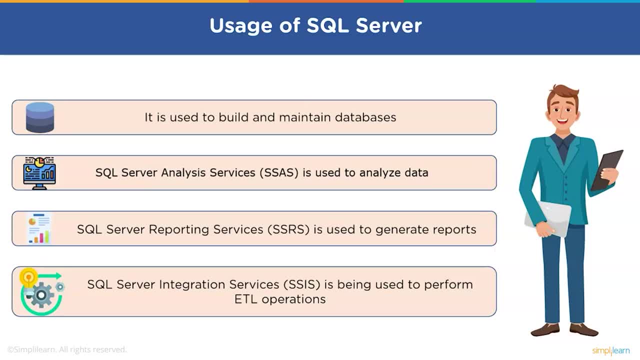 It provides the vehicle for moving data from different data sources to another and changing the data if necessary. The three components in the SSIS platform for starting the data integration processes are: the Import and Export Wizard, SSIS Designer and SSIS API Programming. The Import and 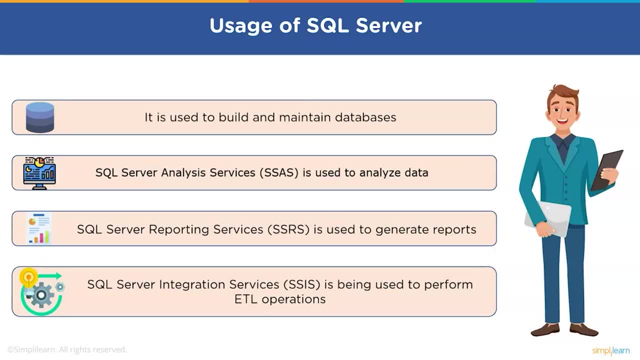 simply transfer data from source to destination, but does not include data transformation capabilities. If the SSIS designer is an integrated component of the business intelligence development studio used for the development and maintenance of integration service packages, SSIS API programming module allows you to code SSIS packages using any number of programming languages. So 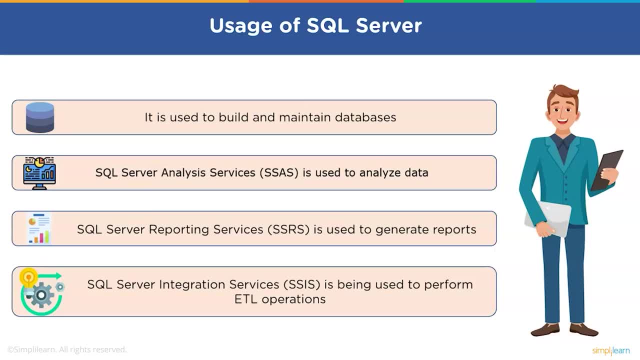 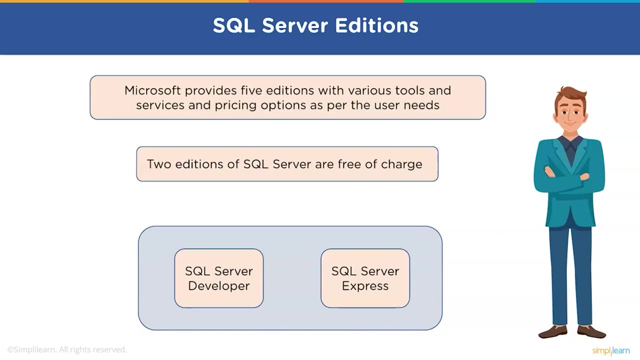 there are lot of features which are available to you In order to manage your data, create your data pipeline structure. it build visualization reports, perform spider web data processing, etc. so it's an enterprise solution. Now let's see what are the different kind of SQL Server. 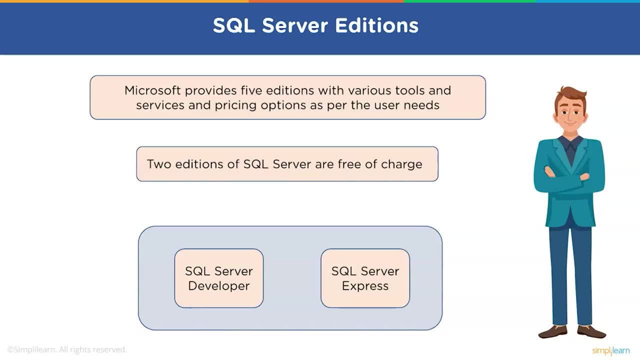 additions. Microsoft procvides five editions with various tools and services and pricing options as per the needs. So the two editions of SQL server which are freeloadedIP- employees, orriters- are available to use If the य or यク Lots of services are available which are free organisation variations. 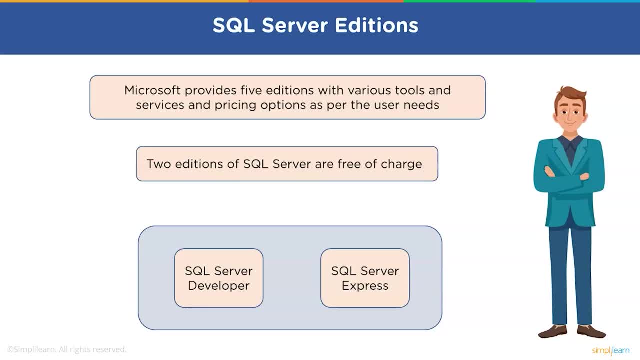 charge are SQL Server Developer and SQL Server Express. Now, the Developer SQL Server Edition works and function exactly like an Enterprise SQL Edition. The only difference is the license is used for testing and development purpose only. This edition is generally used by developers to build and test. 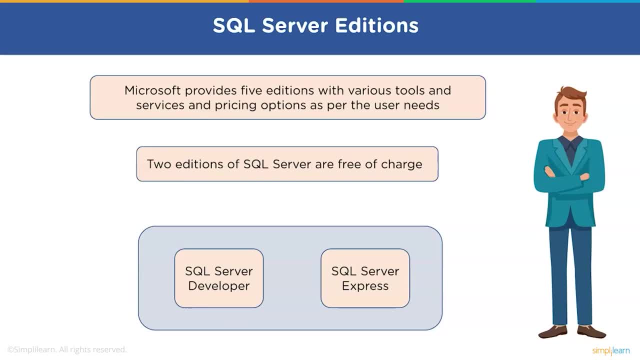 applications on top of the SQL Server, but they can't take it to production. SQL Server Express Edition now is the free entry-level database version and is ideal for learning and building desktop and small server data-driven applications- but not meant for any serious computation- while also having 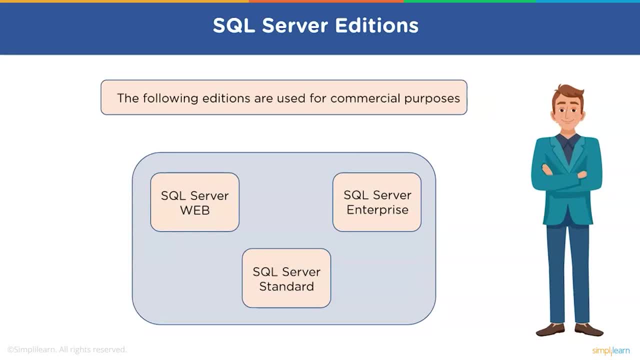 incredibly limited features. Now the other editions are used for commercial purposes. SQL Server Web Edition. It is a low total cost of ownership option for web hosts and web value add providers to provide scalability, affordability and manageability capabilities for small to large scale web properties, as the SQL Server Enterprise Edition delivers. 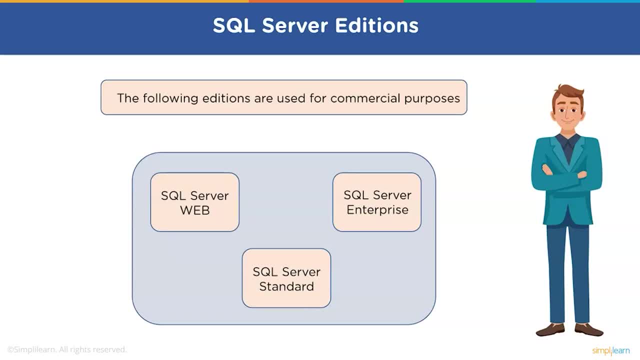 comprehensive high-end data center capabilities with blazing fast performance, unlimited virtualization and end-to-end business intelligence, enabling high service levels for mission-critical workloads and end-user access to data insights. this version has all the features required for big data. now SQL Server Standard Edition. this delivers basic data management and 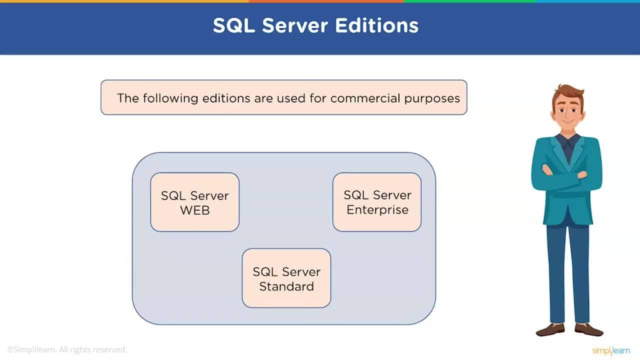 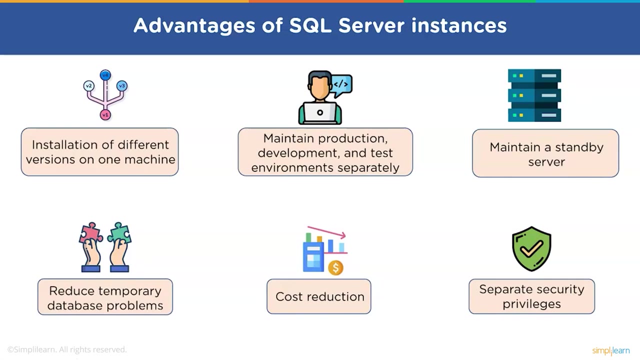 business. intelligent database for departments and small organizations to run their applications and support. common development tools for on-premise and cloud, enabling effective data management with minimal IT resources. now let's look at some advantages of SQL Server instances. its installation is of different versions on one machine. you can maintain different installations. the 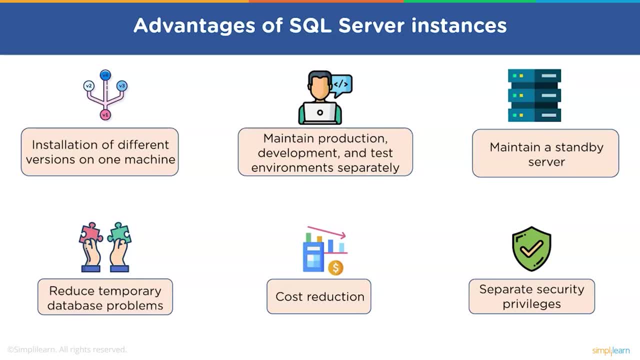 maintenance of production, development and test environments can be done separately. you can maintain a standby server, so installation is streamlined. it can be installed via setup wizard, and the prerequisites of updates are detected and downloaded by the installer automatically. the complexity of the installing the software is minimized significantly. 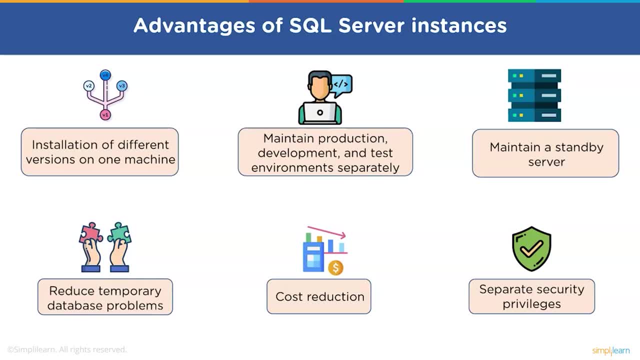 because of automatic installation of updates. other components, such as analytical and database services, can be installed separately afterward. automatic updation also reduces maintenance costs quite significantly. SQL Server 2008 uses policy management to detect security policies that are not compliant, so this feature allows only authorized personal. 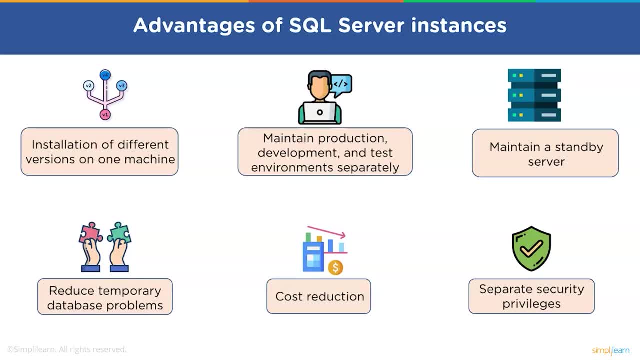 access to the database. security audits and events can be written automatically to log files. MS SQL Server has built-in transparent data compression feature, also, along with encryption. users don't need to modify programs in order to encrypt the data. the MS SQL Server has access controlled, coupled with efficient 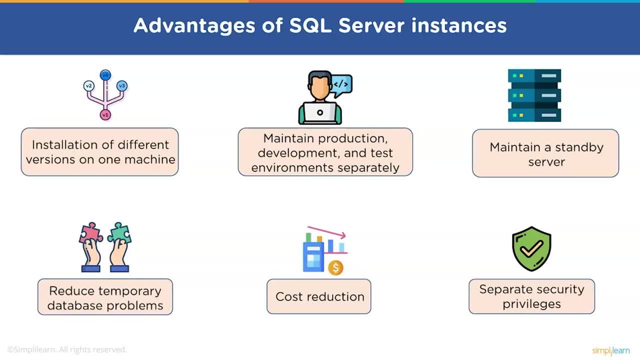 permission management tools. further, it offers an enhanced performance when it comes to data collection. okay, and coming to the cost reduction, so it has lower cost of ownership. SQL server includes effective data management and data mining tools, along with disk partitioning your servers. optimum maintenance can be ensured by 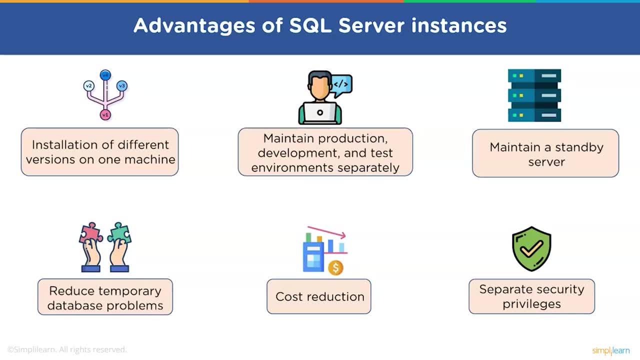 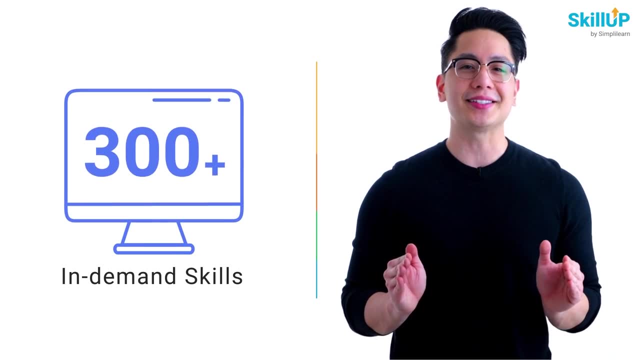 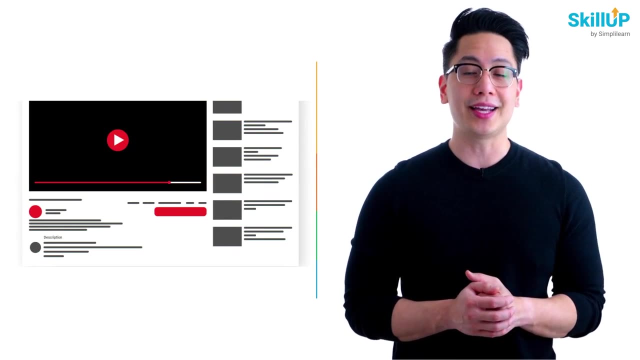 following effective data management practices. these practices also help you ensure the availability and recoverability of data. choose from over 300 in-demand skills and get access to 1,000 plus hours of video content for free. visit skill up by simply learn. click on the link in the description to. 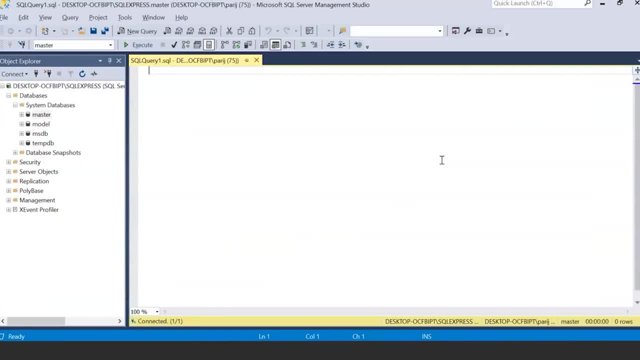 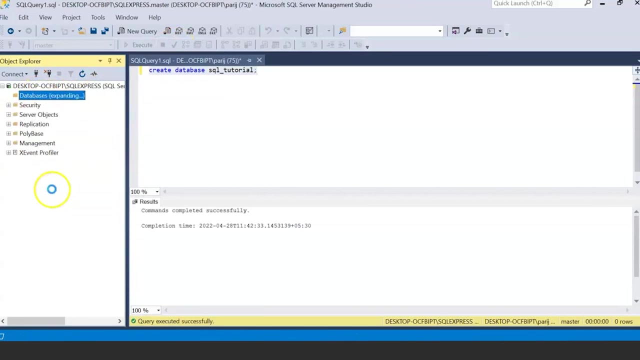 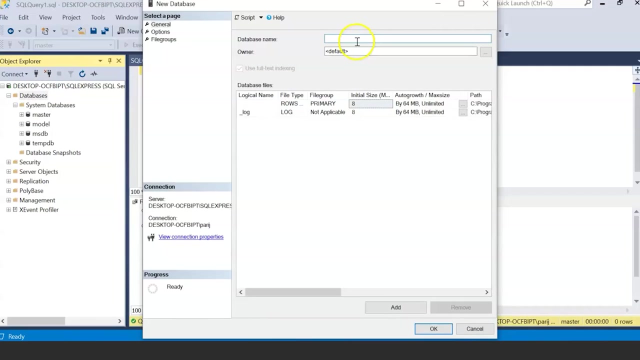 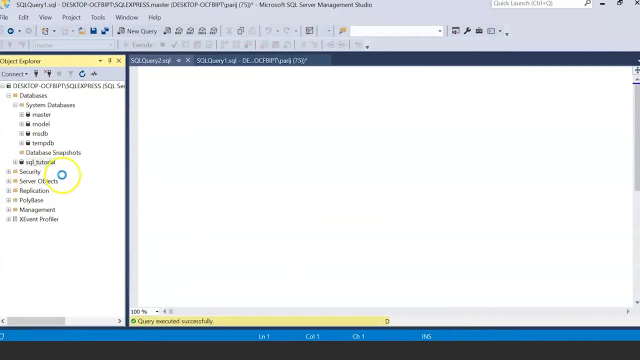 know more. now let's move on to creating a database in SQL server. so I have installed the default SQL Express on my machine and now I'm gonna create a database called SQL tutorial- Traveling Twitter. so let's create a database called SQL underscore tutorial. you okay? now I will write certain queries on top of it. first I'll create a table. 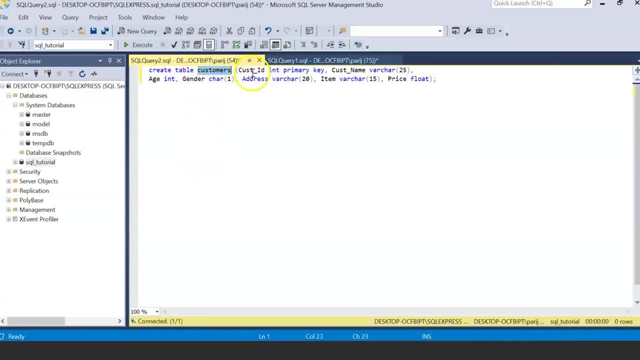 customers. let's create a table customers which has columns: customer ID, which is its primary key, the name which has where care. customer IDs in age, which is an integer gender, male, female. will notify it with one character address, which is generally a large number. string values of will keeping it back at 20, item, which 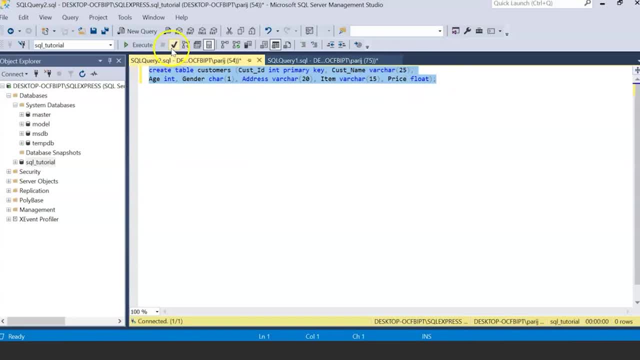 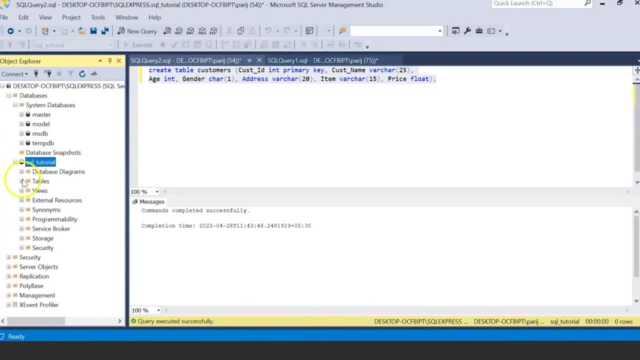 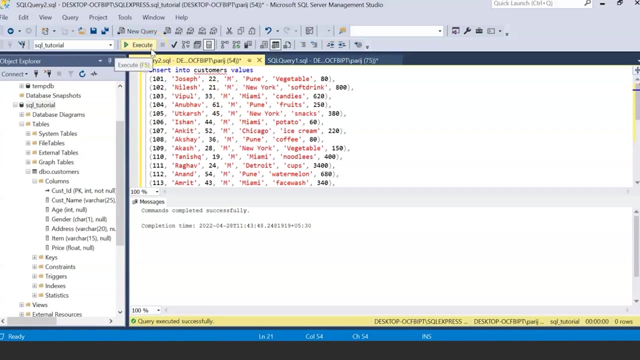 is where care 15 and price. okay, so let's create this table, okay. so now, if you see, this table has been created- DBO curve dot customers. now all the relevant columns which I created here has been present. now I have prepared the script to insert some sample values so that we can query this. 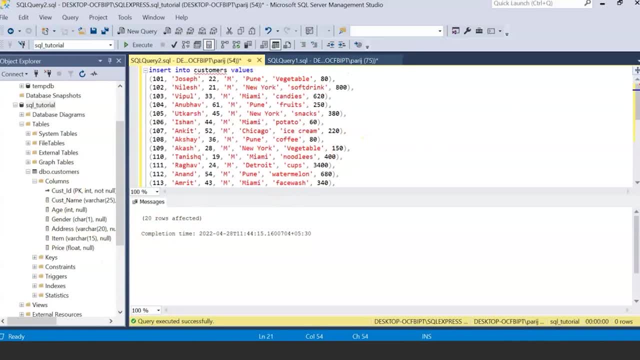 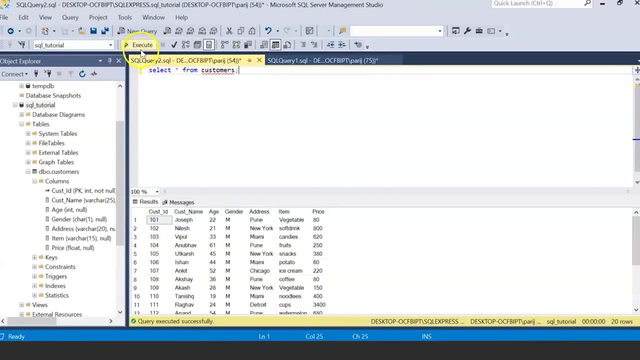 so I have inserted a round above 20 values. so let's just check whether my data is present. I'll do a select star from my customer tables and you can see now the 20 rows with the customer ID: customer name, age, gender, address or name. 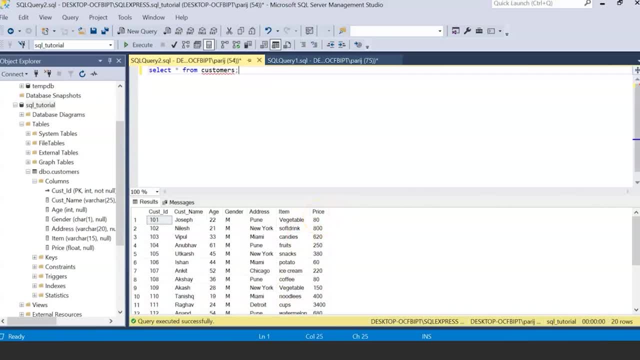 the item which the customer has purchased and the price at which he has purchased. now let me show some variations of the queries which we can perform now. now, select star means you have selected all the columns. I only want to select some selective columns like customer name and gender, so I can. 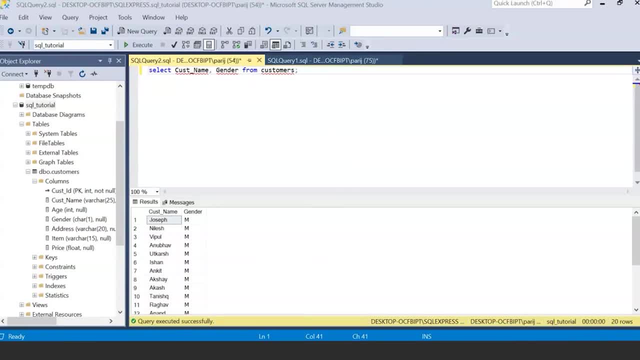 also do that. you just need to give the name of the customer and the gender column. next query: I want to check what is the distinct values of the gender in my customer tables. so I will only get two values, which is male and female. so there is no other value apart from M and F in my customer table. next I have a. 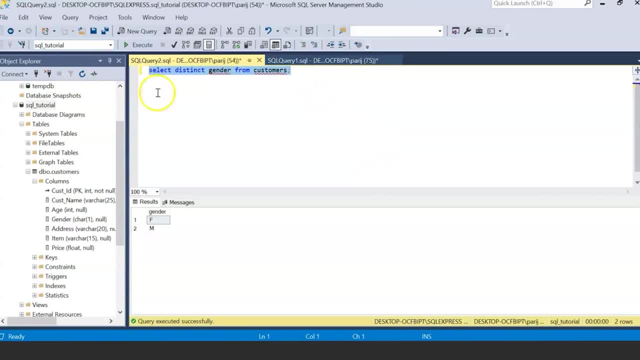 query where I want to find which are: are the customers who have purchased an item. who all are the customers who have purchased an item which is having price greater than 250 rupees? okay, great. so out of 20, only 12 other customers who have purchased a price item which is greater than 250 and? 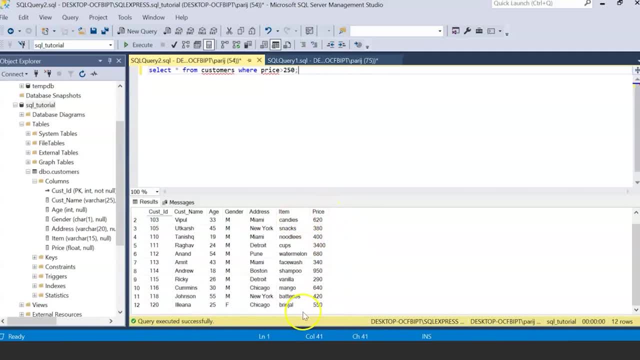 you can see, all the items which are all listed over here are greater than 250. next, okay, I want the customers who are living in New York. okay, fine, I just have to change the where clause where instead of the price. I am now looking at the address, which is in New York. now it is also possible that. 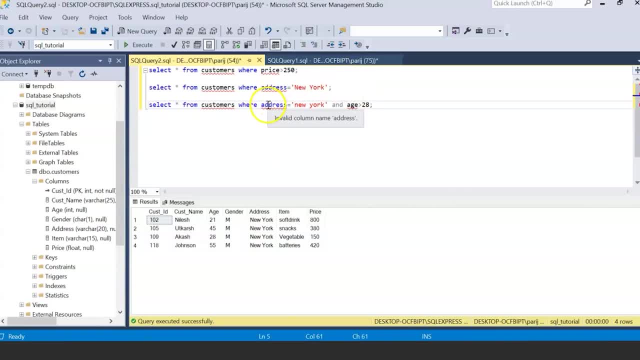 you can apply another filter. okay, people living in New York, but age is greater than 28. perfect, I only have two customers who are living in New York but having age greater than 28, or I want the female customers who are purchasing items greater than 380 rupees. okay, only one out of 20. okay, Elena, now we saw. 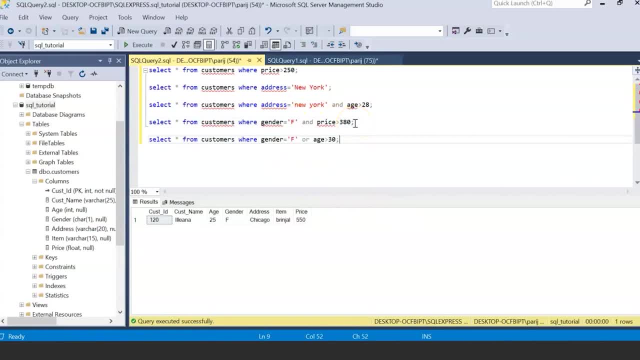 examples of and condition: there is also possibility that, okay, you want female customers or customers who are greater than age 30, so you will get both the records: age 30. age 30. greater than 30, or female customers, both the records will come. or customers who 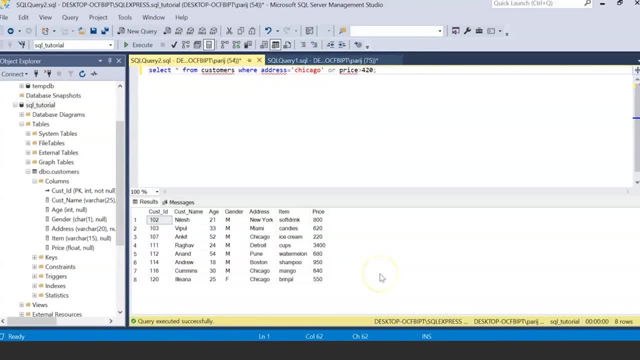 are in Chicago or purchasing items greater than 420. so these are the examples of or conditions. now let's take another example of: not now. I want that the customers who are not purchasing price less than 650, the reverse right greater than 650, so I'll get this answer. or I want the customers who are 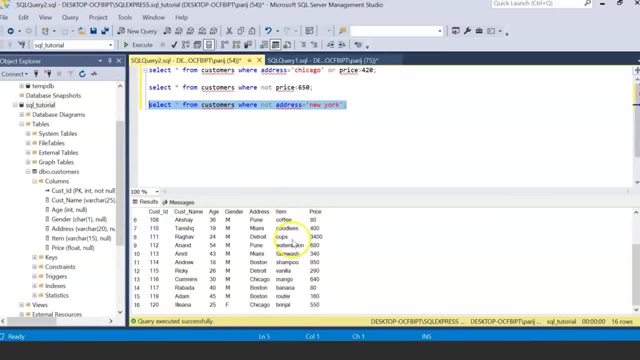 not living in New York, apart from New York, any other address, so all these customers are there, okay, so now these are the examples which I showed. you are the examples where you can play around. you can filter data applying the where clause. now let's take another example of aggregated functions in SQL. now, amongst the 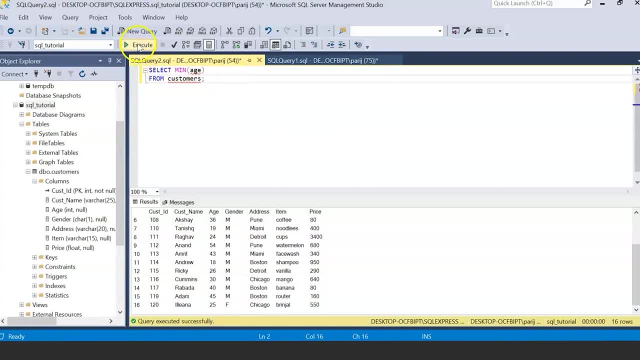 list of customers, the data set of customers which I have. I want to know what is the minimum age of my customer. one of minimum age is 18 years, so one, the minimum age amongst the all the customers is 18 and the maximum is- I can just change it to max- is 61. so the age range 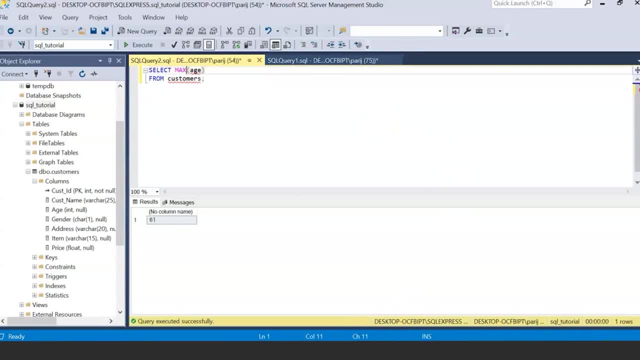 of my customers who are purchasing are from 18 to 61. okay, now I want to know what is the minimum age of my customers. so I'll take one example of aggregated functions and now another example, hypothetical example. I want the average age of my customers where customer ID is greater than 105. okay, so if you see Select star, where 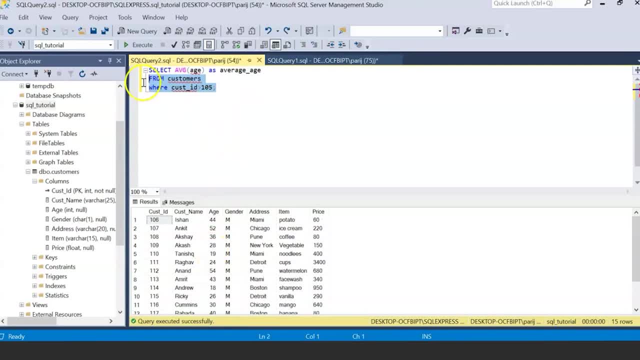 customer ID is greater than 105. I have 15 customers and amongst these, my average age of my customers is 35. similarly, instead of average, I can take the result of the average age of my customers: 35. I want to know the average age of my customers and I will take one example of that. 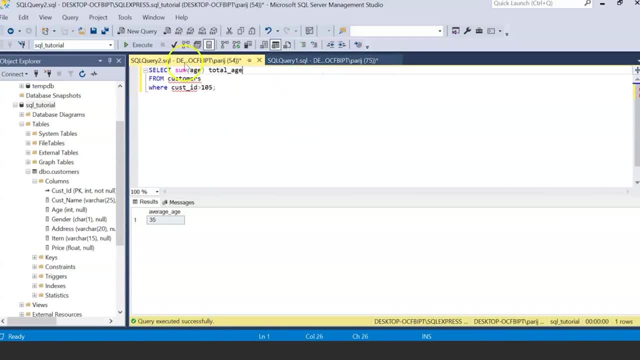 sum total of the age above 105, which is 539 sum total. okay, now I'll show you an example of like. I want the name, I want the customers list where addresses which consists of e letter e in their address, it anywhere in the string beginning in. 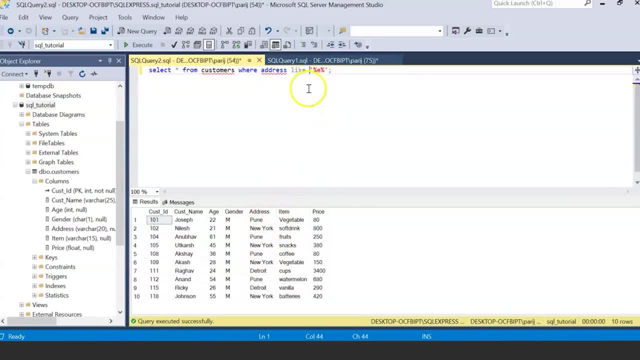 the middle because I have like is a keyword like percentage first. percentage means he can come in any part of the string, okay, and if I just change this example, I remove the percentage from here. it means that I want the customers who addresses end with e, so only Pune will come into the picture, okay. so 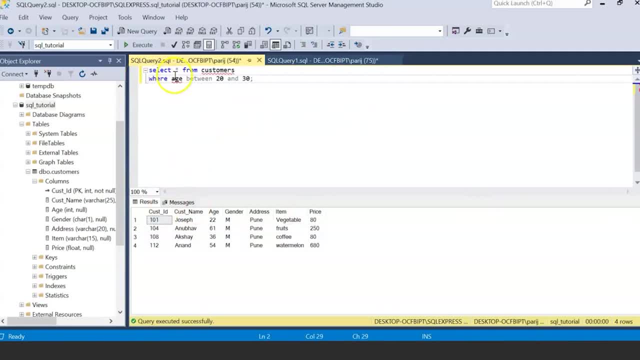 this is the difference. now, coming select star from customers where age which between 20 and 30. so I want all the customers which have belong to age between age 20 and 30 inclusive. so 20 and 30, both are inclusive. so it means the customers which with age 20 and all 30 will also come in. this results in: 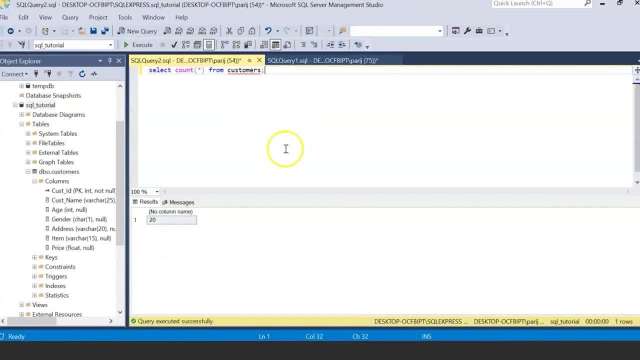 next example: I want the count of total customers. in my data set, which is two, 20, I inserted 20, so I know now I have 20. I want the count of male customers. oh, out of 20, 19 are male. okay, great, and if I group by, now let's see an example of group by. so I 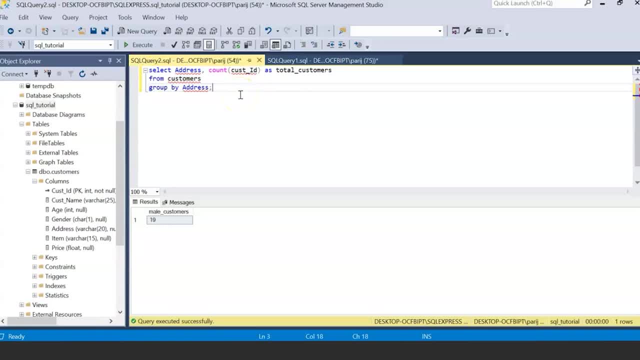 want the count of customers grouped by address. so how many are living in Boston? how many in Chicago, Detroit, Miami, New York and Pune? so I have a customer wise total count. total basis the address group by. okay, so it's a very important concept. you can group by any. 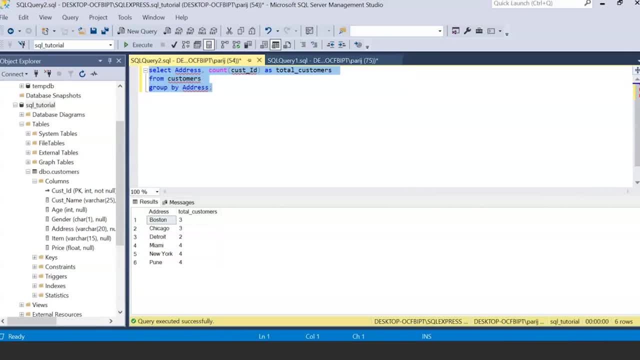 column and then you can do a measure, count, a count, a sum, an average. you can do any aggregated calculation basis the other columns which are not in the group by. like. another example, I want an average age per address. so in Boston the average age of my customer is 34. 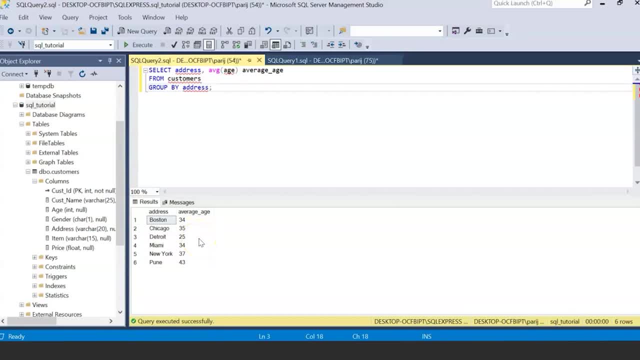 who are purchasing items: Chicago 35, Pune 43, so like that you can do some analysis. this is all data analytics. now let's see another example. I want to. I want to filter data now after doing a group by. it's not so, please note, this is different from where clause in. 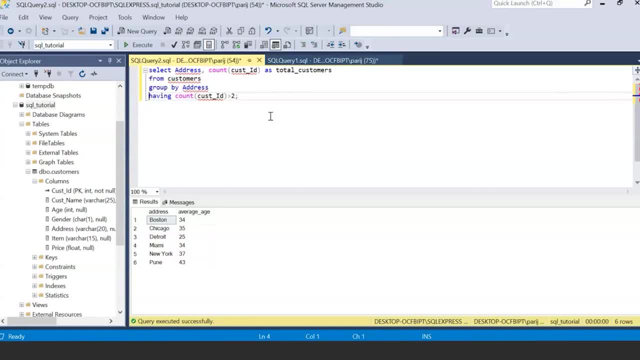 where clause means filtering data before grouping, having clauses used once you want to filter data after grouping. so you are doing a group by address, Count of customers and then only those cities should come where count is greater than two. okay, so the customers, the only those addresses are listed where customers count is greater. 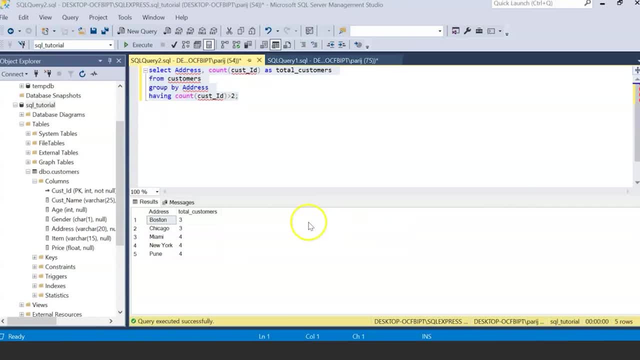 than two. okay, now this is an example of inner queries. you want group by customer name and age: only those customers having age Greater than the average age of overall. okay, so my average age, if I say my average age from customers- is 36, so overall all the customers which are more than 36 should come over here. 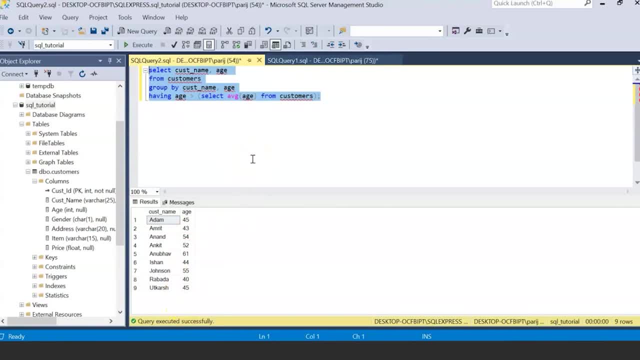 listed over here and that's what is up. okay, now let's talk about order by. it's like sorting. you want to order by address, so it has ordered by, by default, b, c, d, m, n, p, which is ascending, and if you apply keyword descending, so it will do the reverse way. similarly, I can order: 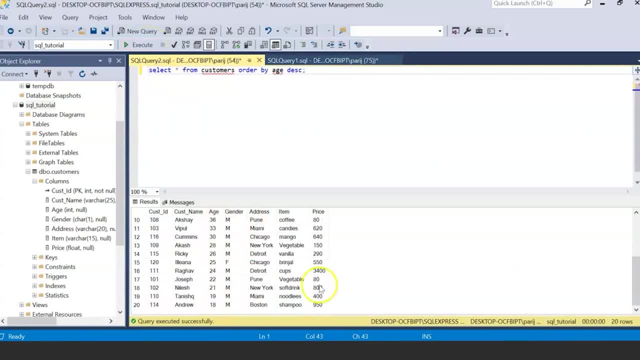 by age, which is descending: highest age first, lowest below. or you can do order by multiple columns, where order by address, By address descending, and then same address. within the same address the customers should be ascending. addresses are descending, but within the address the customer names are sorted in ascending fashion: a first, b, c, d, like that. now there's an inbuilt function. 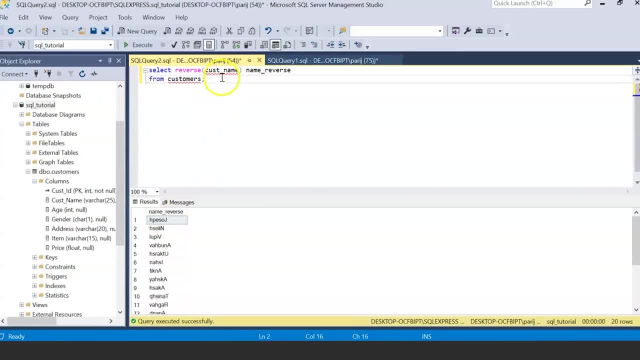 in sql server: reverse. if you see, this has reversed the name of the customers. it's in reverse fashion. okay, the characters are reversed. another example is where you are now. this is not on the table, this is just a sample query, where you are replacing vegetable with 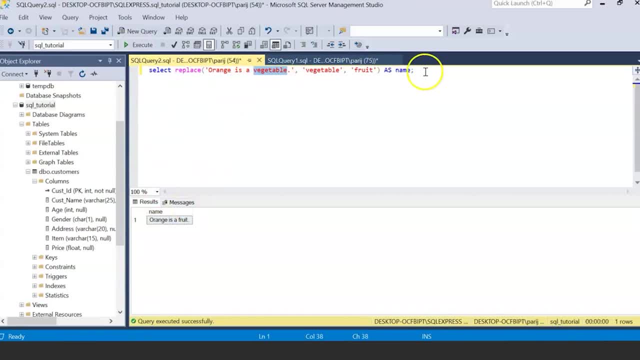 fruit. so orange is a fruit. you have replaced vegetable with the fruit. it is just a. you don't need a table. you can just also write such queries where you don't need a table. okay, then there is a function called l trim, which is which will remove. 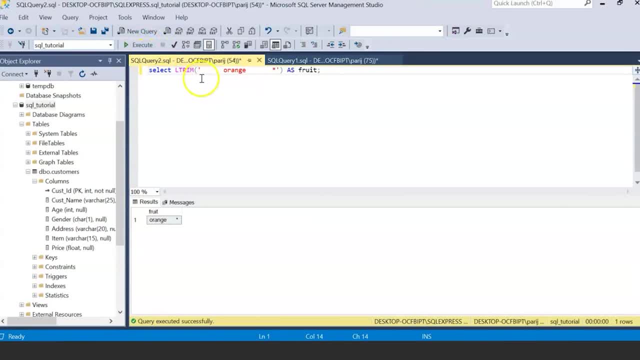 all the blanks from the left hand side. r trim, which will remove the blanks on the right hand side. okay, let me read an: r trim, it will remove the blanks on the right hand side. and then there is trim function, which will remove from both the sides, left and right. now let's. 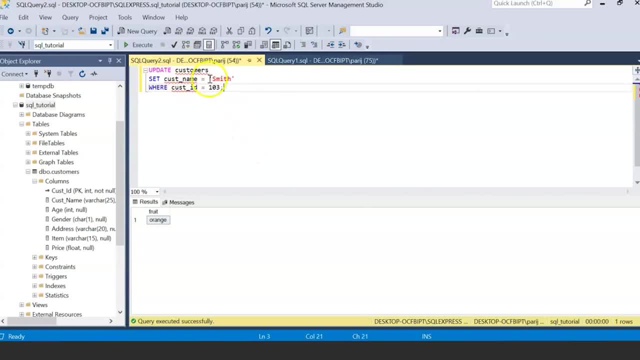 take an example of update command. i want to update the name of my customer whose customer id is one zero three. first let's check what's the name. so customer name right now is whipper. so i'm going to update the name of my customer whose. 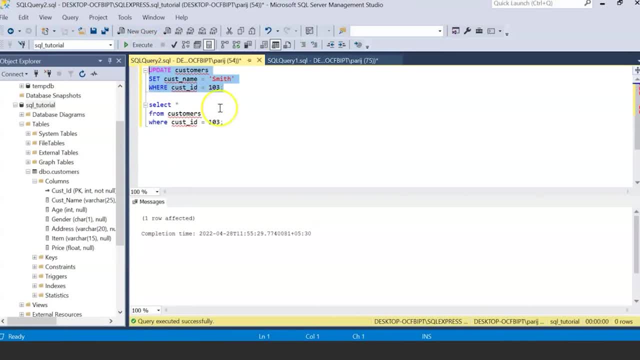 customer id is one zero three. so this is an example. i want to change it to smith and if i re query, it is changed to smith. okay, so this is an example of update. now, if i want to delete, let me check who is at one zero one. i want to delete customer one zero one, joseph. i will delete it and now. 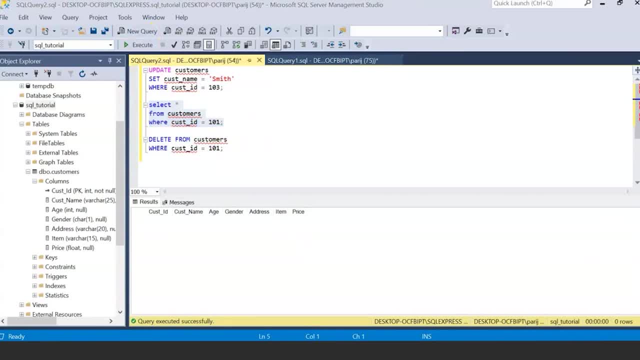 if i want to check. okay, there is no customer at one, zero one. okay, now let's take one other example, another example of inbuilt function: ascii. it will give you the ascii code of the character ascii a, ascii four, etc. etc. right, so there is n number of possibilities. there's a n number. 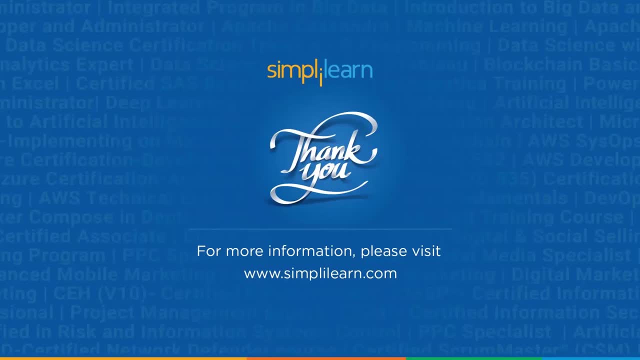 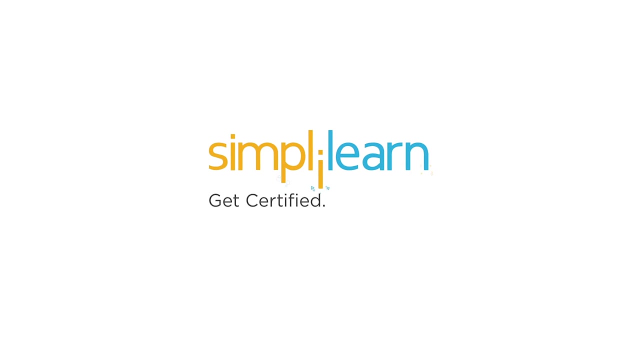 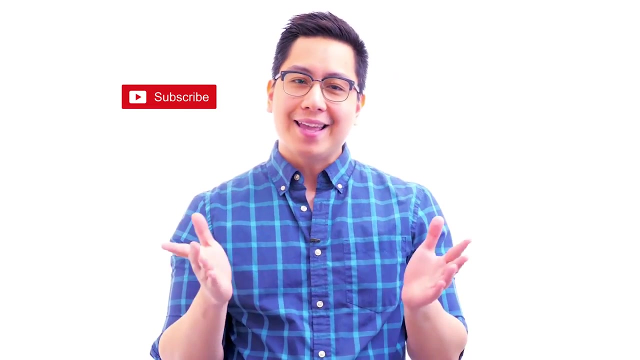 of queries which you can write, but this is just a glimpse and basic understanding of for you to get started with sql queries on sql server. i hope you all had a great learning session and i hope to meet you in my next session. thank you, hi there. if you like this video, subscribe to the simply learn youtube channel and click.